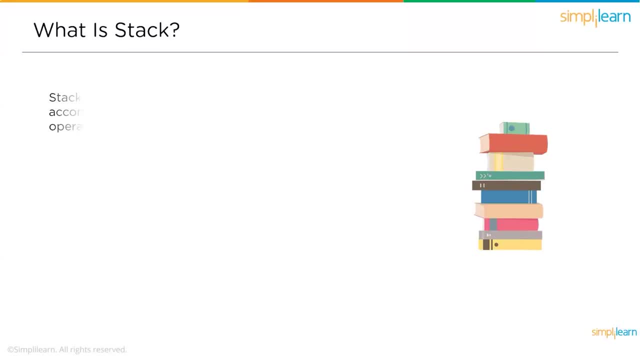 What is a stack? So, basically, stack is a linear data structure, just like arrays and linked lists. The only difference is that it follows a specific order when an operation is implemented on it. So what is the specific order that it follows? That is, LIFO, Last In, First Out, or 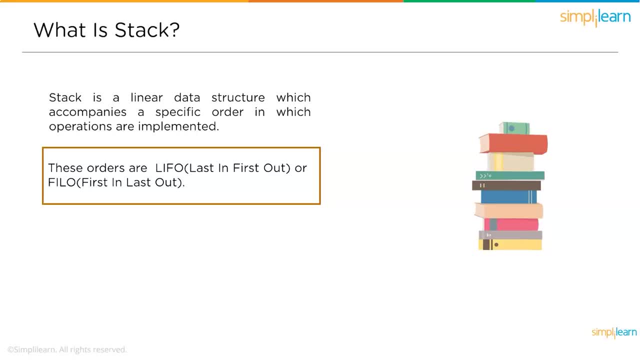 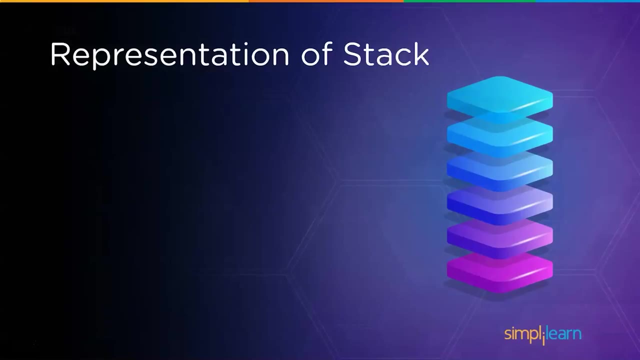 FALO First In Last Out. In the next part we will understand this order in a much better way. All operations can be done only at the one end of the stack, that is, on the top. Now we will discuss much about that in the operations part of the stack. Now let us understand. 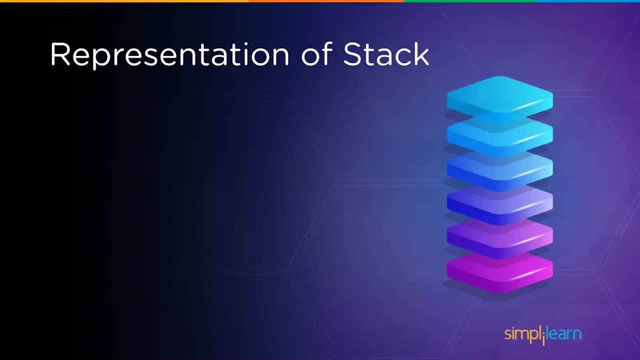 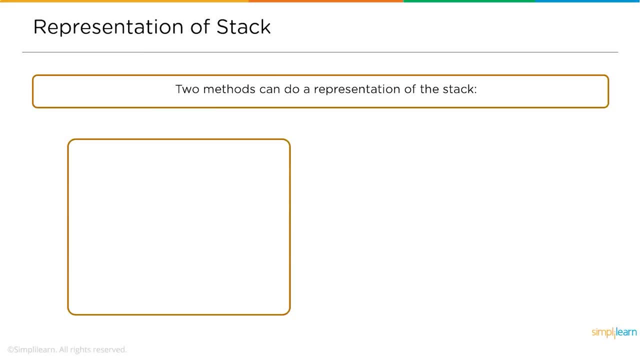 the first fundamental, that is, the representation of stack. That is, how do you represent a stack normally? So a stack can be represented using two different methods, That is, using an array or using a linked list. So in an array, we will be using the. 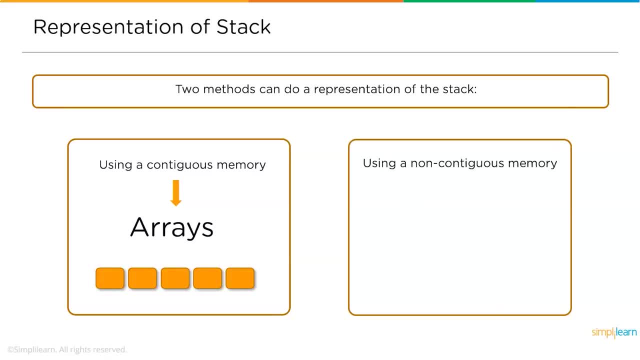 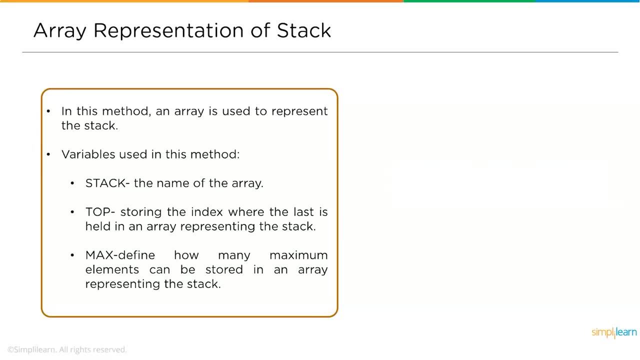 continuous memory And in stack we will be using a non-continuous memory and the stack will behave like a dynamic stack or a dynamic data structure. Now the first method, that is the array method. So in this method an array is used to represent the stack, As you. 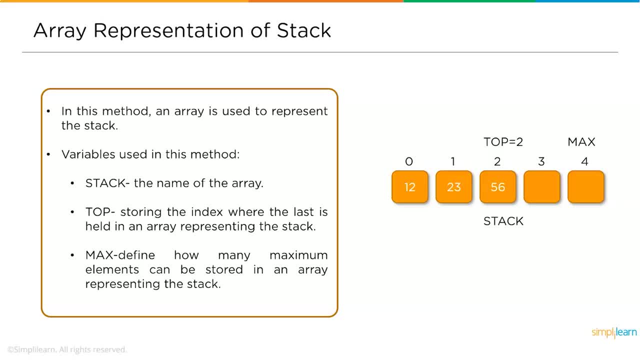 can see in the image below, we have a stack, So the name of the stack is stack itself, And you can see two more things here. that is, top is equal to two and max is four. So the max is the value of the array or the length. 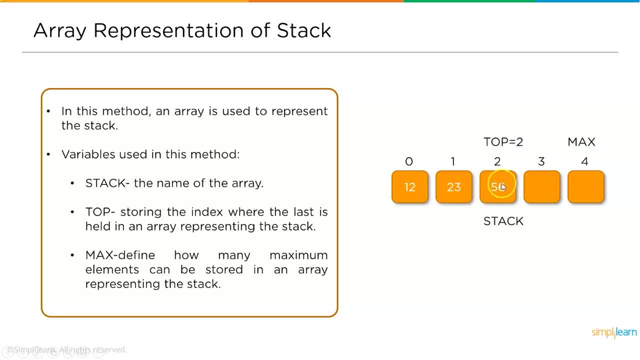 of the array, The maximum length of the array, and top is the position where the last element of the stack is present. Here, in this case, 56 is the last element in the stack and top is inclined or it is addressing to that particular address, that is, two. 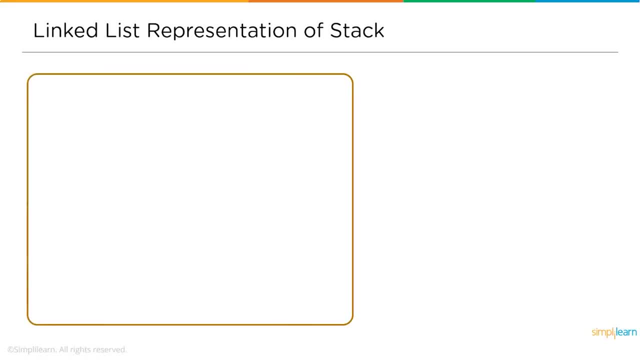 And now let us discuss about the linked list representation of stack. So in this method, a dynamic data structure, that is, a linked list, is used to represent the stack. This representation leads to a dynamic stack. It does not need to define the maximum number of elements present in the stack. 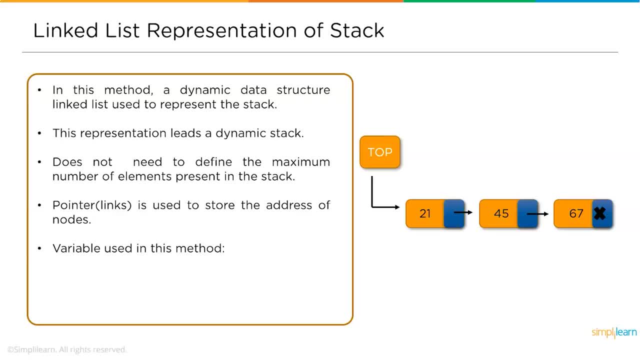 Remember, in arrays we had to define the max value. In the previous example we had the max value as five, but in here you need not to assign the max value as the stack itself as dynamic. The pointers links are used to store the address of the upcoming nodes and the variable used. 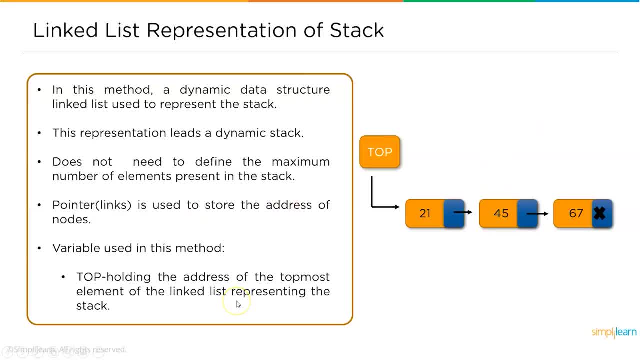 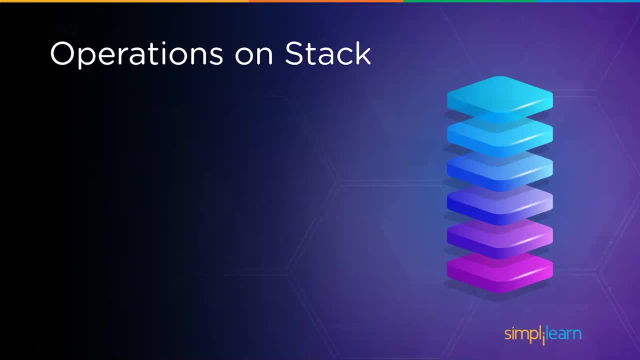 in this method is top, So the top is holding the address of the top most element in the linked list representing the stack. Now, moving ahead, we shall understand the basic operations on stack. Now here we will understand the previously discussed definition, that is, push, pull, etc. 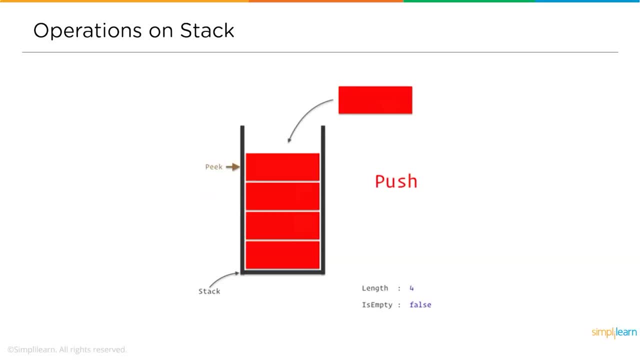 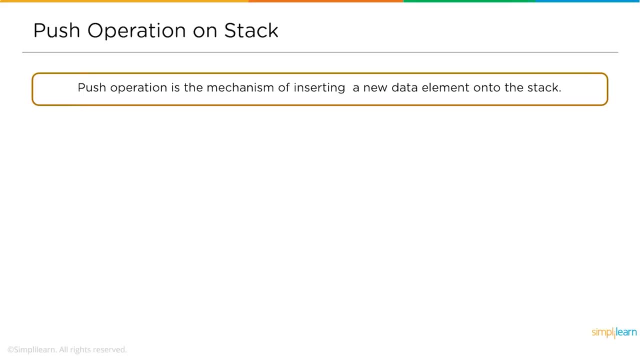 in a much better way. So the basic operations on a stack are Push, pop or pull and peek. Now let us discuss each one of them in a detailed way. The first one is push operation. So the push operation is the mechanism of inserting a new element into the stack. 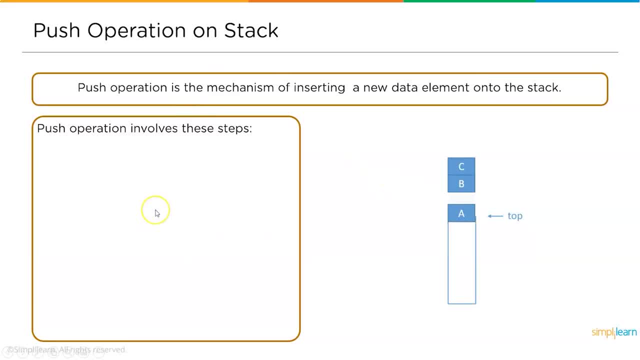 As you can see, we are trying to insert the elements from the top. So the push operation basically involves the following steps: Check if the stack is either full or not. So basically, whenever you are trying to insert an element into the stack, you need to make: 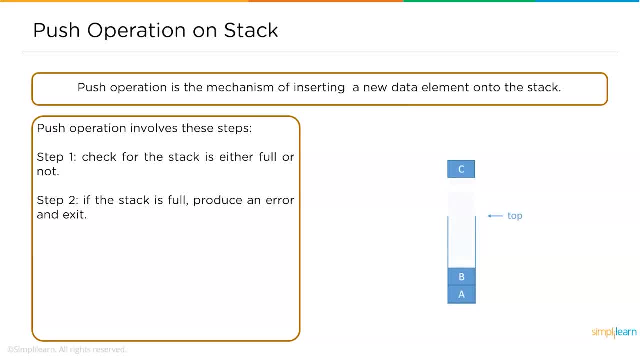 sure that the stack is empty Or It has some space. If it is full, you cannot insert an element into the stack. Step 2. If the stack is full, produce an error and exit. That is what I was talking about. 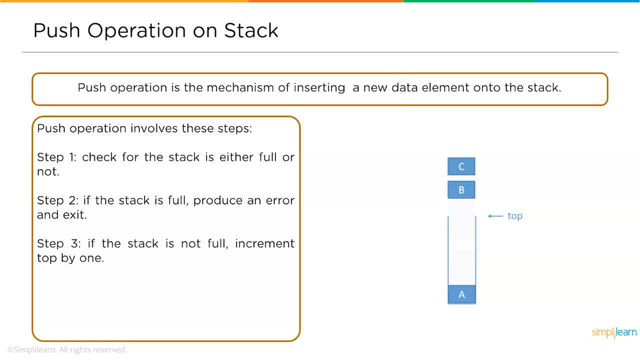 Now the step 3.. If the stack is not full, increment the top by 1. That is, when you are inserting an element, then you need to update the top value. For example, in the previous slide, when we had the array representation of a stack, we 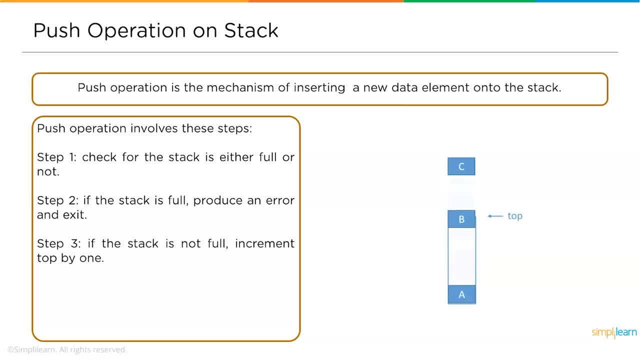 had the top value as 2.. So if you try to include an element into the stack, Then you need to update the top value from 2 to 3. That is incremented by 1.. Now the 4th step: Add data elements to the stack where the top is pointing. 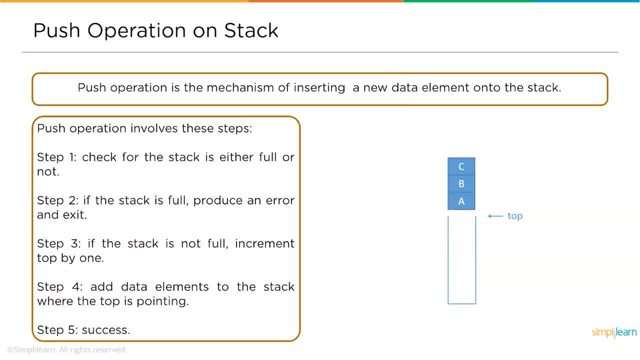 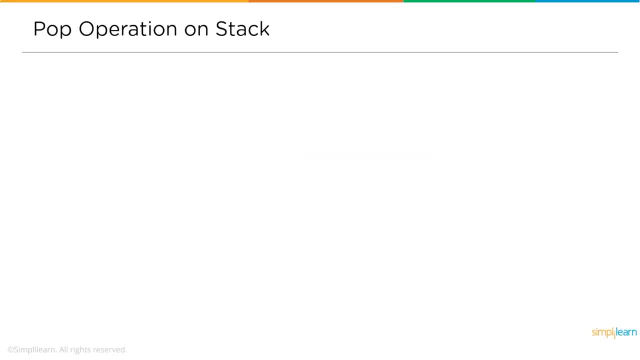 And finally, 6S: The push operation has been successful. So this is how you insert or push an element into the stack. Now, followed by push operation, we have POP or PULL. So the POP operation is a mechanism of eliminating or deleting elements from the stack. 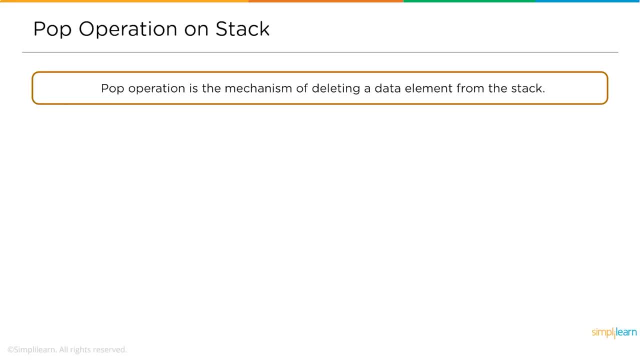 So the POP operation is a mechanism of eliminating or deleting elements from the stack. So the POP operation is a mechanism of eliminating or deleting elements from the stack. So the POP operation is a mechanism of deleting or removing one data element from the existing stack. 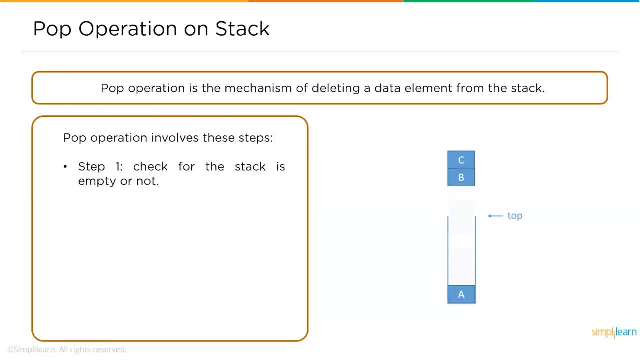 So we shall understand the POP operation in a much more detailed way. The operation involves checking the stack is empty or not. If, in case, the stack is not empty, then you can carry forward the POP operation. But in case if the stack is empty, then you have to provide an exit status and exit the. 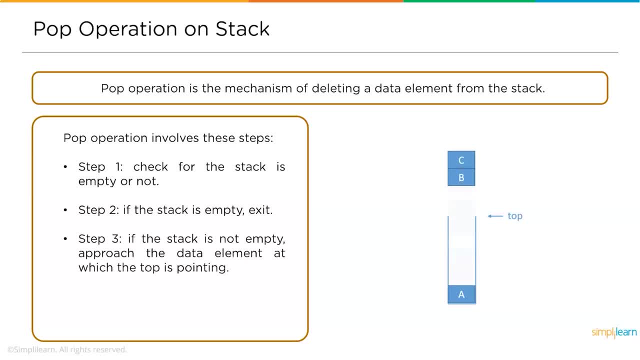 control and leave the stack. So If the stack is not empty, approach the data element at the top that is at the top position. for example, in the previous array example, remember right- we had the top position pointing towards 2.. 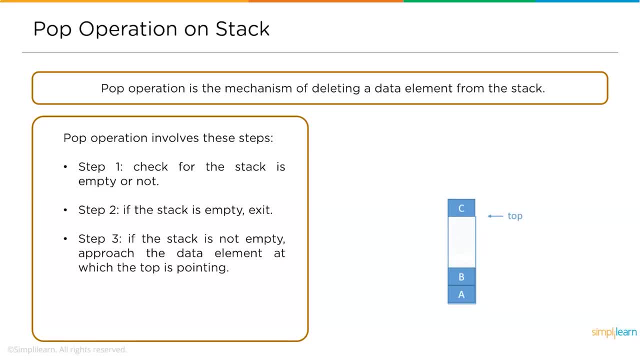 So you need to take the control to the top position and pick out the element and POP And finally decrease the top by 1.. So when you eliminate the top element, then the top value from 2 will be decremented to 1.. 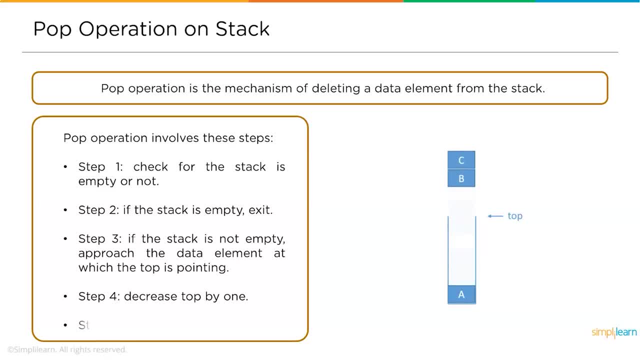 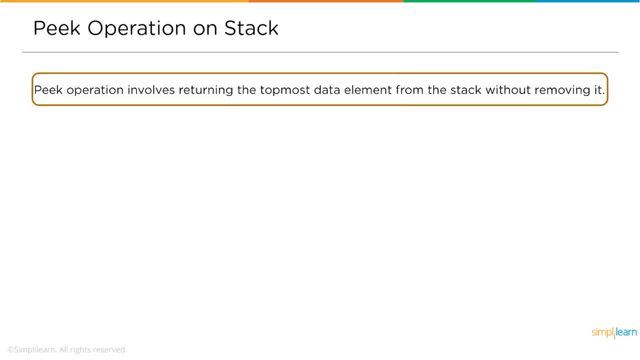 So this is how the POP operation is carried over on a stack. So if the stack is not empty, approach the data element at the top, That is, at the top position. Next one is the PEEK operation. The PEEK operation involves returning the top most data element from the stack without 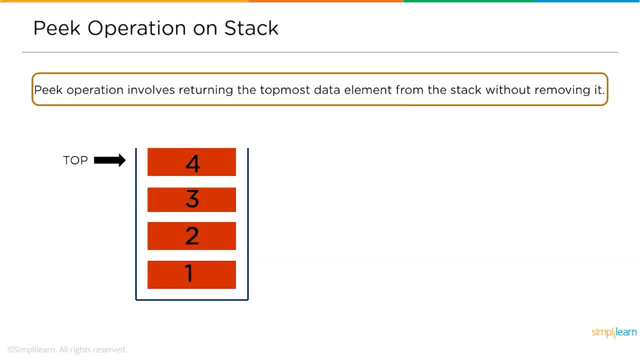 moving it. So here you can see, the top is pointing to the element number 4, and you're PEEKing the element number 4 and you're not removing it from the stack. You're just returning the top most data element. You're passing the value of the top element. 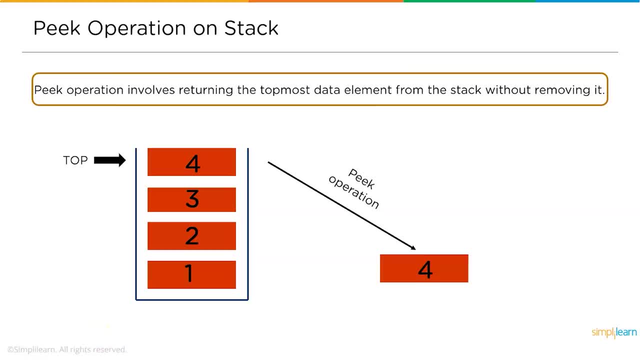 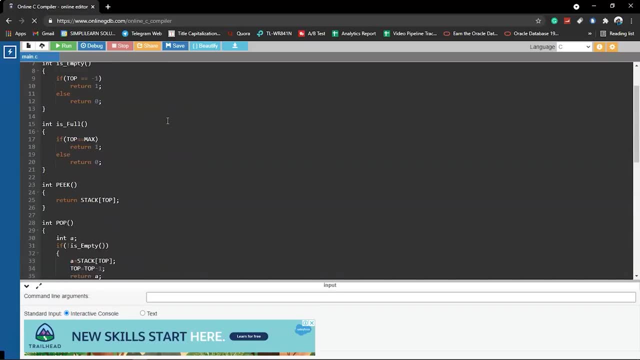 So, So to understand the push, pop and pick operations on stack in a much more better way, let's carry out a practical example. Now we are on the practical mode and here you can see on my screen, we have the code example for the stack. 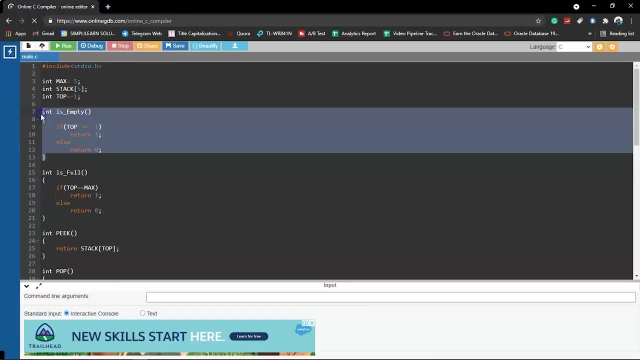 Now. first we will be checking if the stack is empty, as per the steps mentioned in the previous discussion. we will check if the stack is empty or not. If it is empty, then we will return, else we will continue. and again, another step: we also. 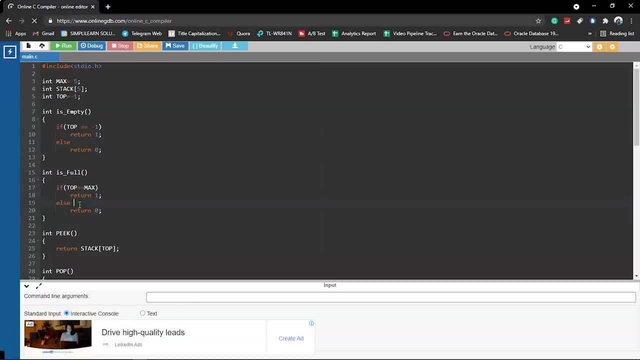 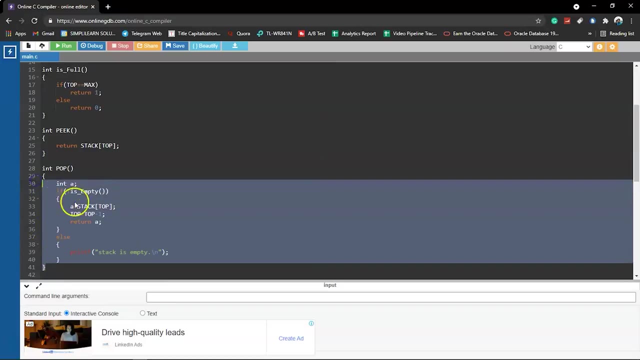 check if the stack is full. if the stack is full, we will exit, else we will continue with the operation, whatever it is: pick, pop or push. And here we have an example for the pick operation that we discussed previously and followed by that we have a pop operation. we are trying to exclude an element from the stack and another. 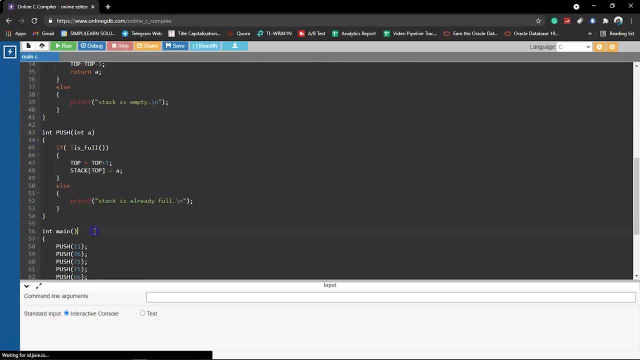 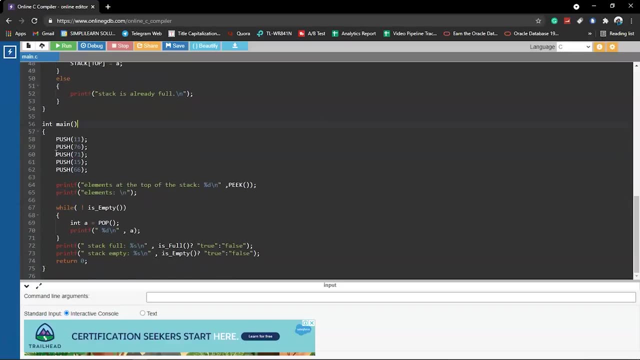 one. we have the push operation where we will be trying to push the elements into the stack. So these are the three functions for push, pop and pick. Now we will try to push in the elements And also pop and try to involve some functions on it or run some operations on the stack. 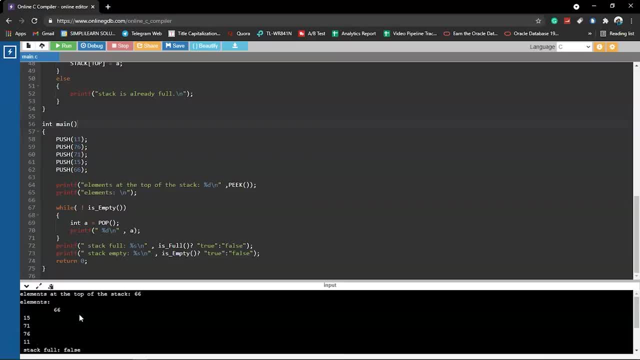 Now let's run this code and see the output, So you can see that the code has successfully executed. and we have the statements here. The first one says: the stack is not full. that is false. and stack is empty. that is true, right. 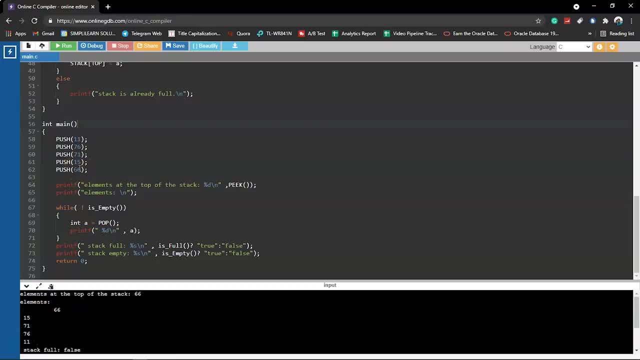 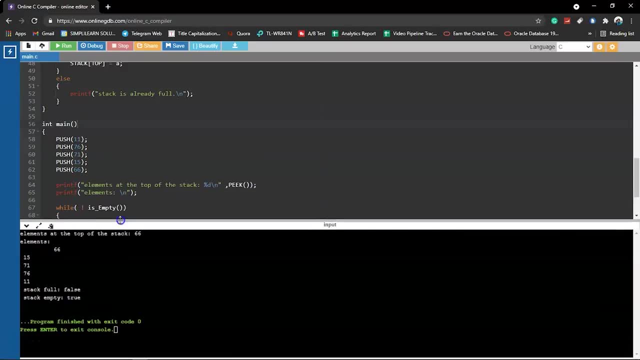 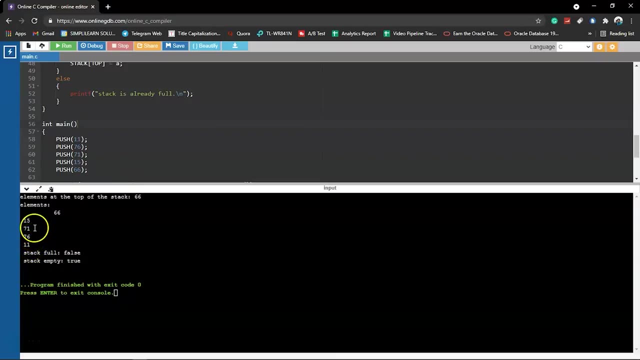 And after that you can see that the elements which we tried to push into the stack, that is, 11,, 76,, 71,, 15 and 66. are been pushed into the stack And, if you clearly observe it, we have the element 11 in the bottom 76 upon that 71. 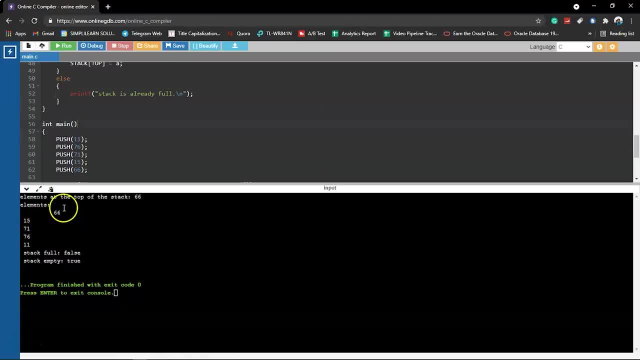 upon that and 15 and last 66. So the order is first in, last out. that is, the first element was pushed first, and when you are trying to eliminate the elements from the stack, then you will first pick out 66, followed by that you will pick out 15.. 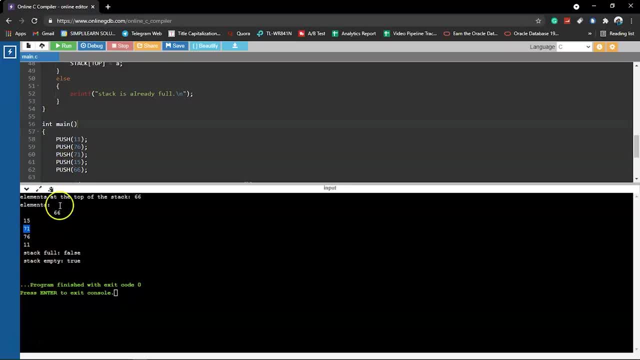 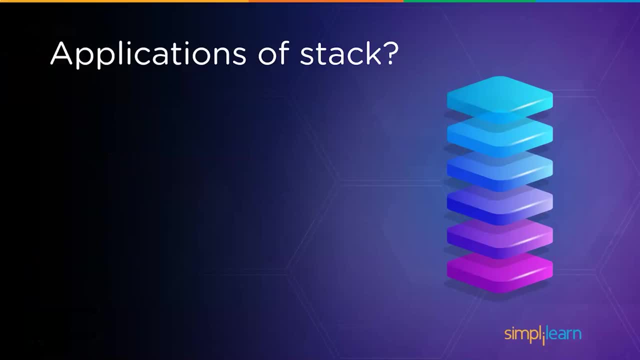 Followed by that. Then you will pick out 71 and so on. So this is the rule: what stack follows? Now, I hope I made myself clear with the example. Now we shall continue with the applications of stack. So these are the few applications of stack. 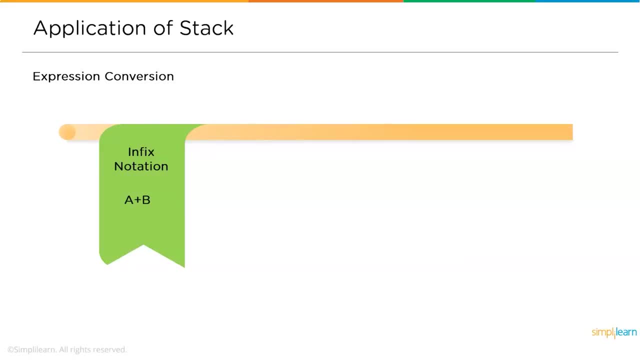 The first one is expression conversion. So you can see, we have the infix notation, prefix notation and postfix notation. So the infix notation is no rocket science. There is only one thing here to learn, that is, we have two operands, A and B, and we have 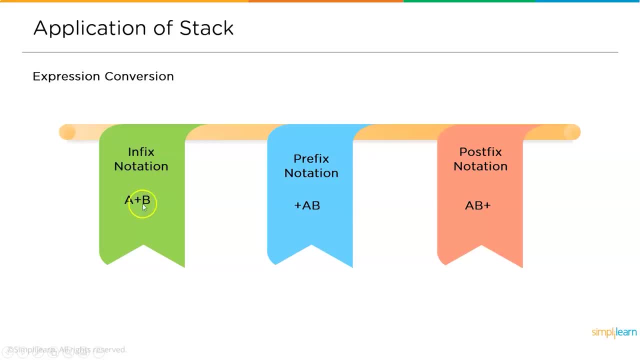 one operator, that is, the addition operator, in between those two operands, And when you use the prefix notation you will have the operator located at the first place, Then you will have the operands followed by it, And in the postfix one you will have the operands first and followed by the operands. 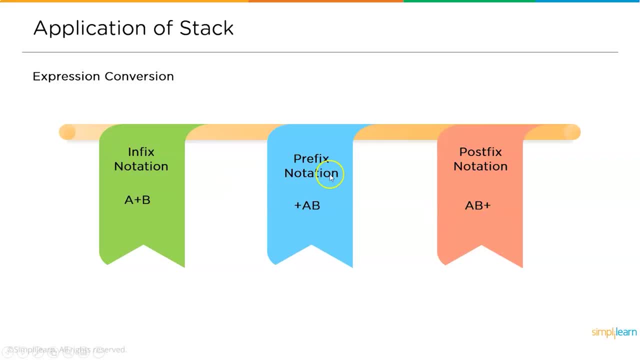 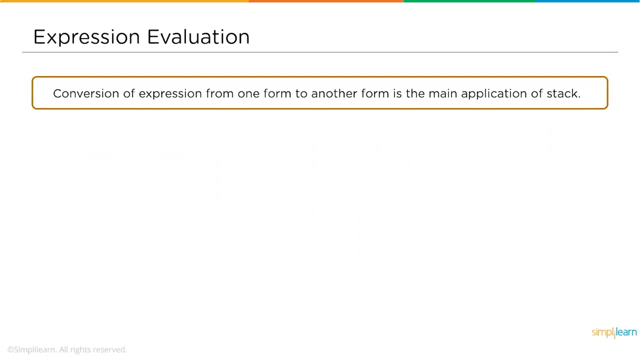 you will have the operator. So basically, all the infix, prefix and postfix notations give out the same results, but the only difference is the representation of those operands and operators. Now let us understand this in a much more detailed way. So conversion of expression from one form to another form is the main application of 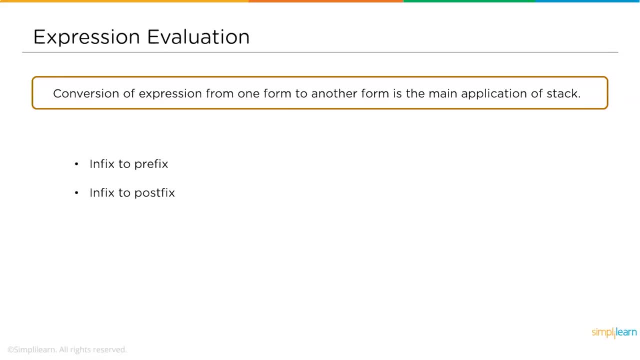 stack. So we have the first one, that is, infix to prefix and infix to postfix. Now let us see an example. Here you have 1 plus 2 star, 3 plus 4.. So this is the normal infix notation, And when you try to present the same expression in the form of prefix notation, 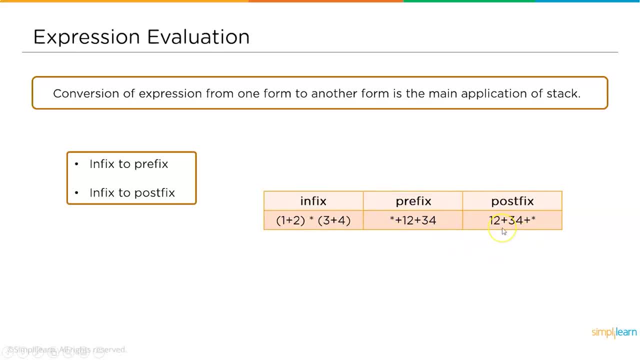 So this will be the result, And this is the result for postfix. The next one: prefix to postfix and prefix to infix. And this is the way you write the prefix notation. And if you want to convert that to infix, this is how you can write it. 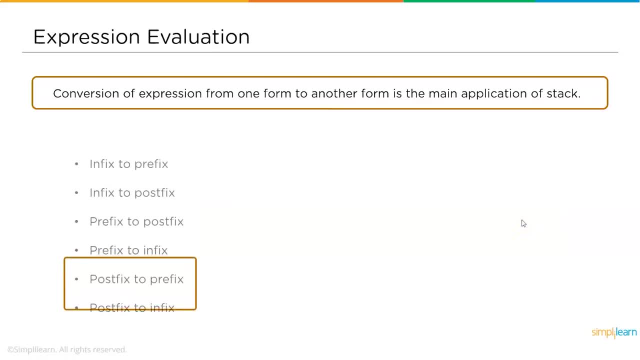 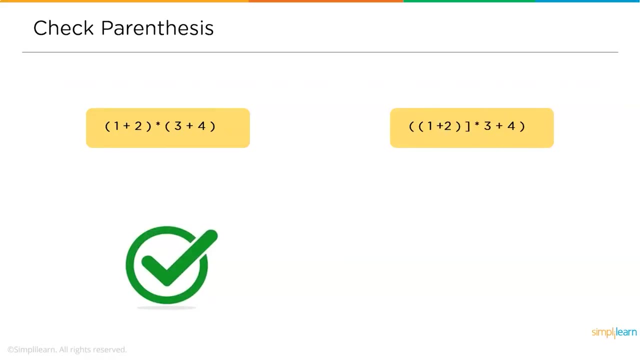 And this happens to be the result of postfix notation. And finally postfix to prefix, postfix to infix And these are the results Now, followed by expression evaluation. The next important application of stack is checking parenthesis And you can see if the parenthesis is set properly. the expression gets evaluated. 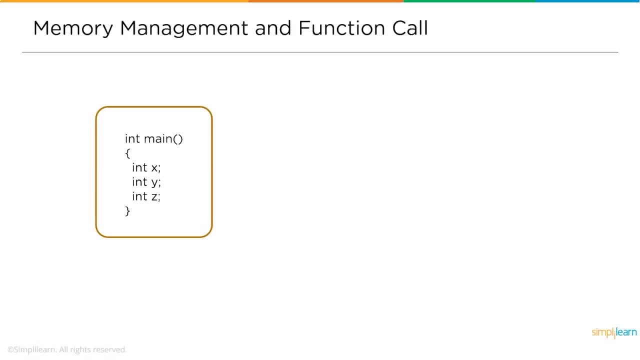 If not, it will not be evaluated. Now the last one: memory management and function call. The very useful thing of using a stack is the memory will not be allocated to your stack elements unless the function is called. Here You can see it is the main function. 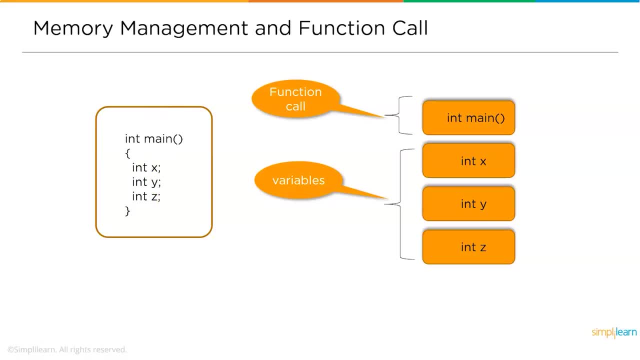 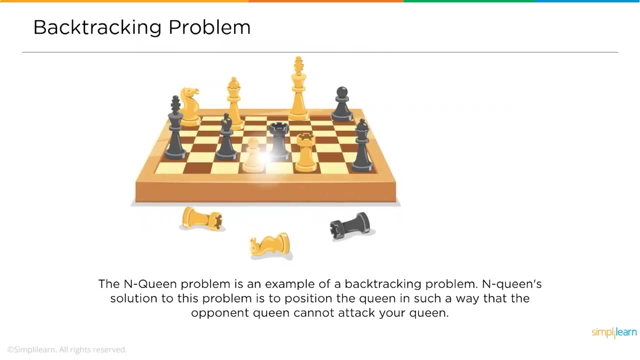 And these are the elements that you wanted to declare into your stack, And unless you make a function call, the elements will not be declared their memory Or the elements will not get the memory allocated for them. Now, another good application of stack is the backtracking problem or the nqueen problem. 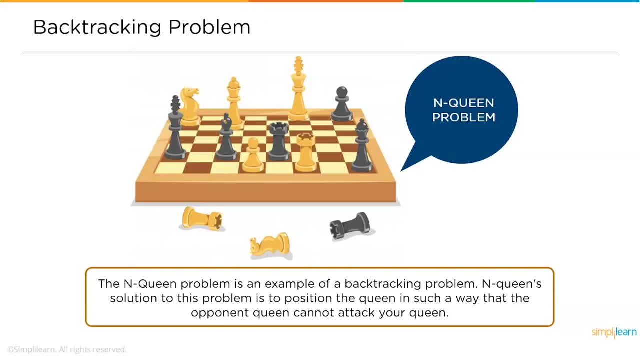 The nqueen problem is an example of backtracking problem. The nqueen solution to this problem is to position the queen in such a way that it will not be declared, And this is the main function, And these are the elements that you wanted to declare into your stack. 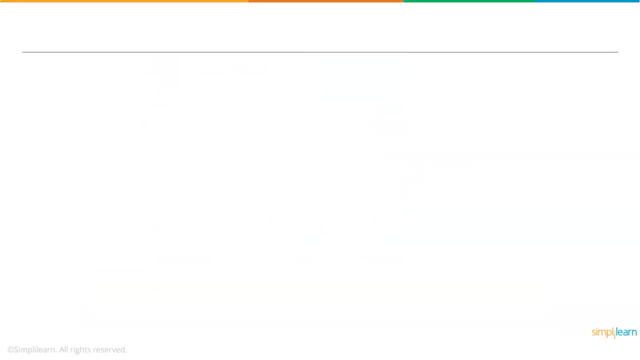 The opponent queen cannot attack your queen Now. another example is string reversal. You can see on my screen we have a string that is A, B, C, D and E. Now, using stacks, you can reverse this Right. 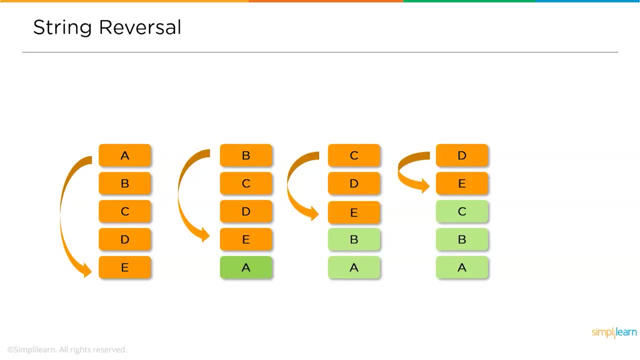 So you're basically eliminating an element and relocating it to the first place And finally, after reversing your string, this will be your result: A, B, C, D and E. Followed by that, we have conversion evaluation. 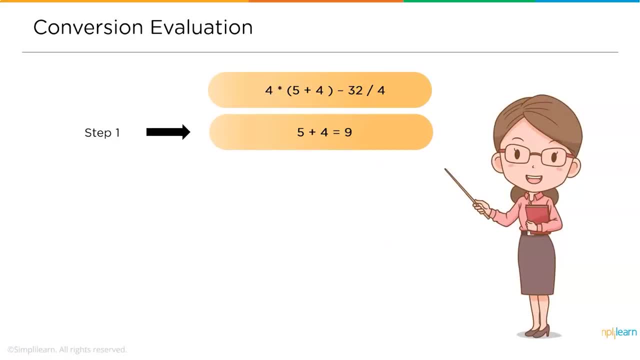 So stack is used to evaluating the expression as shown in the example. Since parenthesis has the highest precedence, 5 plus 4 gets evaluated first, and it will result in 9. Then multiplication and division have the same precedence. Now the associativity comes into picture. 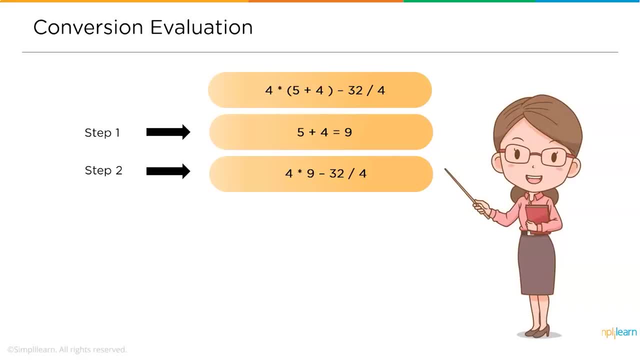 So the associativity is always from left to right. So first 4x9 will be executed, which will result in 36. And then 32 divided by 4, which will give us 8.. Now we have 36 minus 8, which will give us an answer that is 26.. 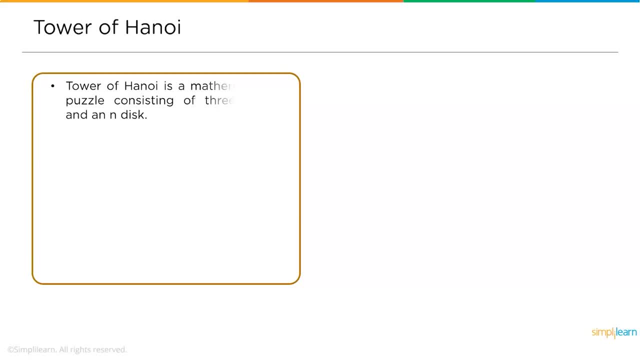 Now the last application is the Tower of Hanoi. So the tower of Hanoi is a mathematical puzzle consisting of three rods and N disks of some rules. The first rule states that one disk can move only at a time. The second rule is that 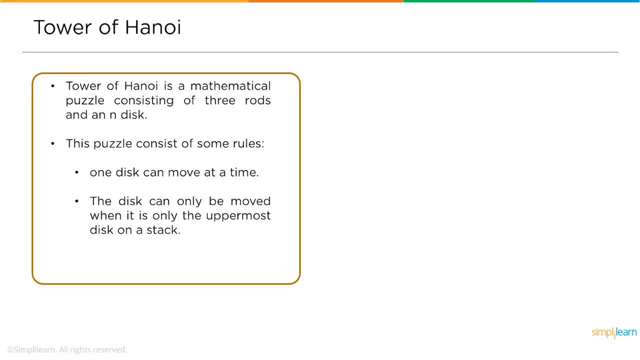 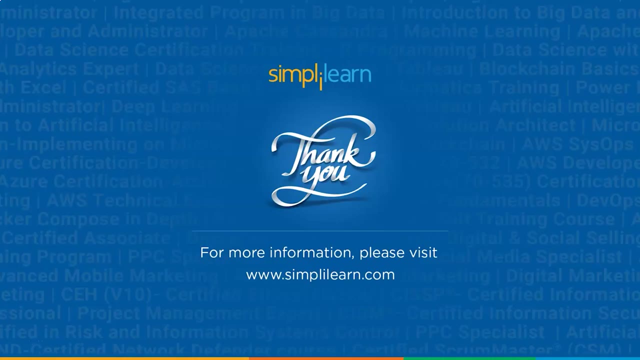 the disk can only be moved when it is at the uppermost position on the stack, The third one: no disk is allowed to place on the top of the smaller disk. So this is how the Tower of Hanoi works Now. with that, we have come to an end of this tutorial. 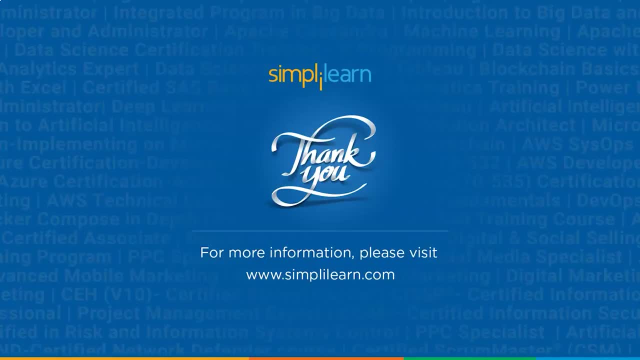 on stacks. If you have any queries regarding the topics covered in this tutorial, or if you're looking for the code executed in this particular tutorial, then please feel free to let us know in the comment section below, and our team of experts will be happy to solve all your queries Until. 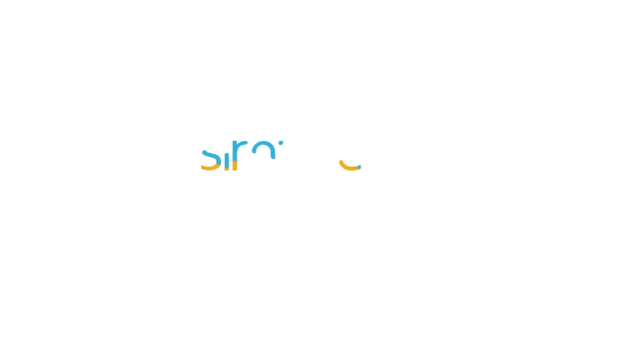 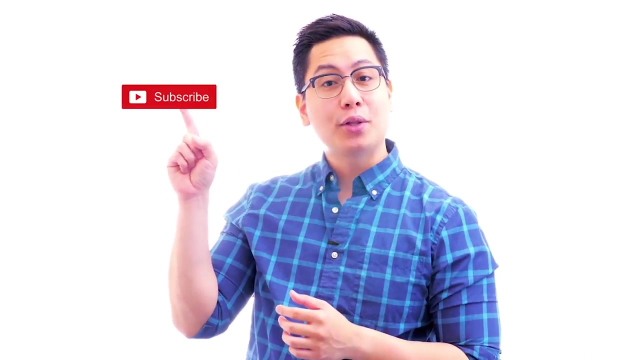 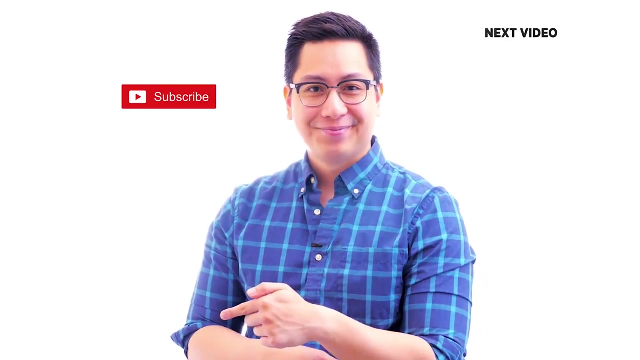 next time. thank you, stay safe and keep learning Hi there. if you like this video, subscribe to the Simply Learn YouTube channel and click here to watch similar videos, Turn it up and get all the latest updates. To get certified, click here.